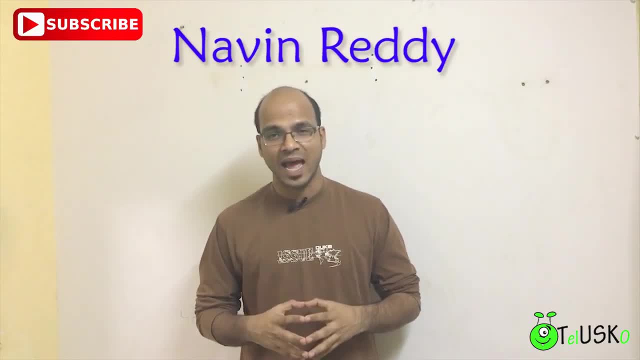 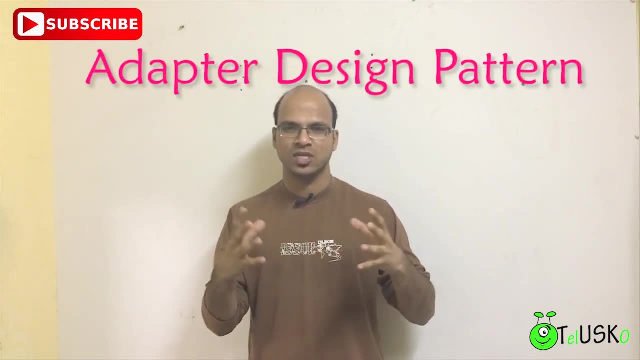 So welcome back, Aliens. This is Navin Reddy from 30 Squad Learnings, and in this video we'll talk about adapter design pattern. Now this is: this is the one of the design pattern we have used in Java, So we have already seen a video on design pattern side. So approximately we have 23 design patterns. 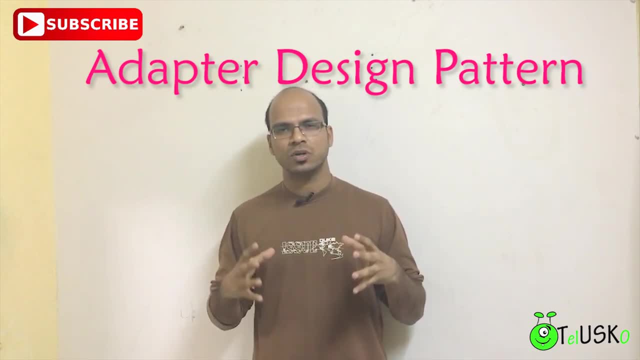 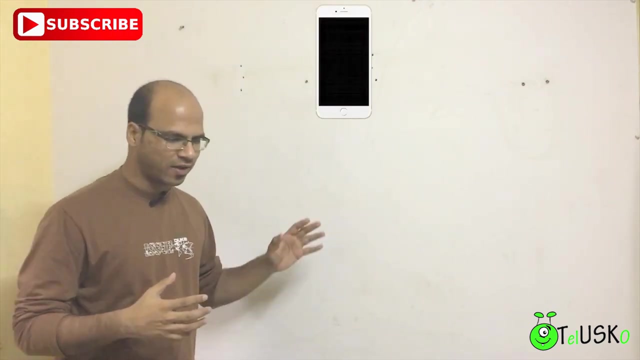 and there's one of them. Now, this is a part of structural design pattern. Now, basically, how it works. So let's imagine. so let's imagine an adapter. What is adapter now? So let's say you have an iPhone 6.. Okay, you have. let's imagine you have an iPhone 6 here and in this iPhone 6, you 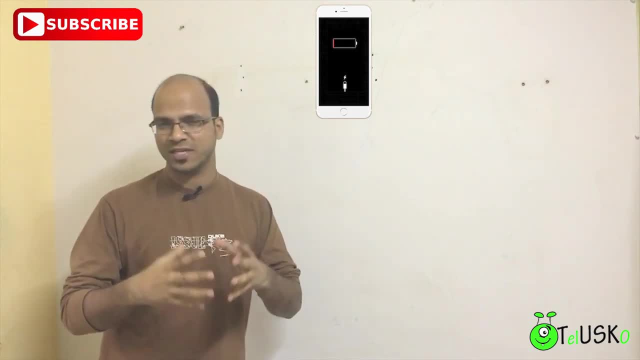 have. you want to charge this phone now. So you went to your friend's place and now you want to charge your phone. Of course, you require a charger right and unfortunately you forgot your charger at your home. Now you are asking your friends to give you the charger of iPhone 6.. Now he is using 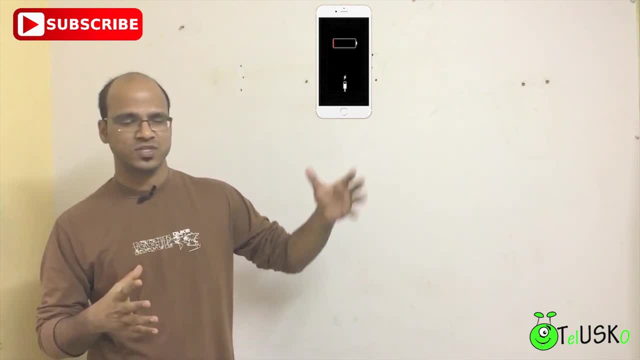 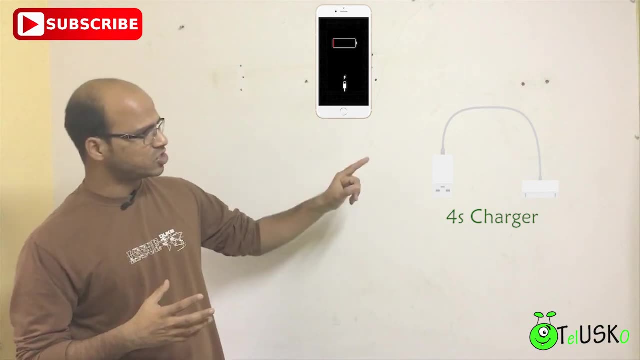 iPhone 4s, right. So now you'll be having a charger for iPhone 4s, which is that? Now, how can you charge with iPhone 6 with the help of iPhone 4s? Because iPhone 4s charger is a bigger charger. They have a bigger slot. What about iPhone 6?? We have a small. 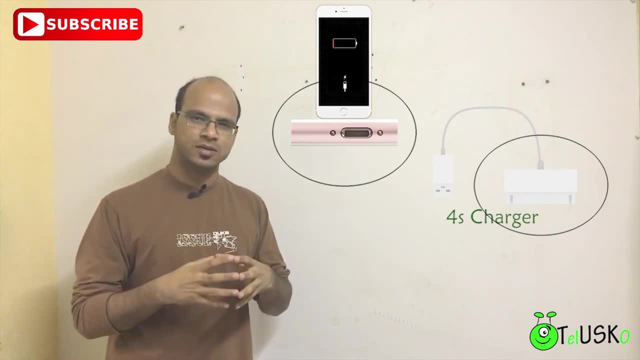 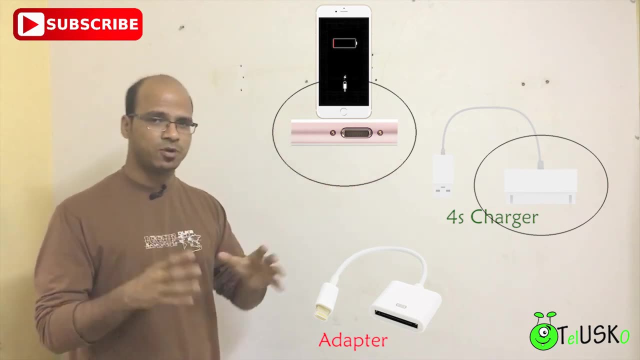 slot. Now how to charge this? So what we need? We need an adapter here. So what if you can just use this adapter to combine or to charge your iPhone 6 with a charger? Is it possible? Of course, if that, if that adapter works, it will charge your phone, right? So that is what adapter is right. 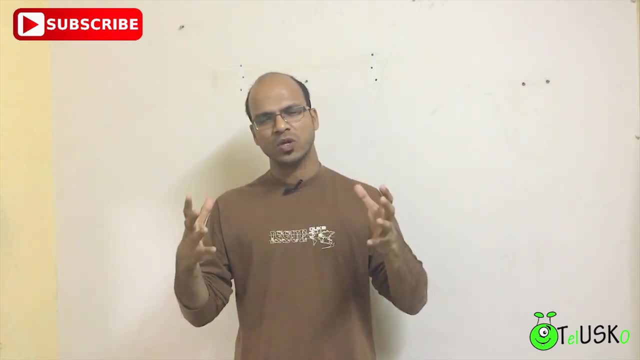 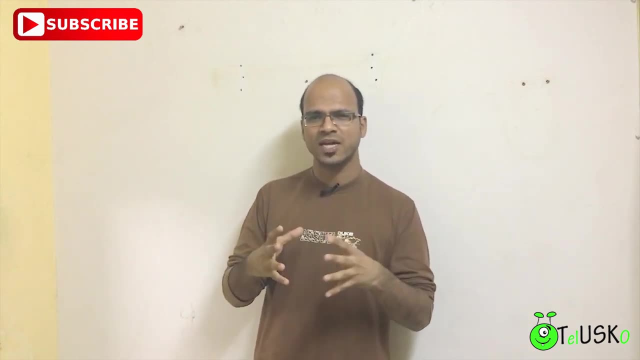 So that's your adapter design pattern. But how to include this in Java? right, Because we are in a software world. This is hardware. How can you include that in a software world? So now let's imagine, for that we'll go for a different example. We'll not take the phone example in the practical. 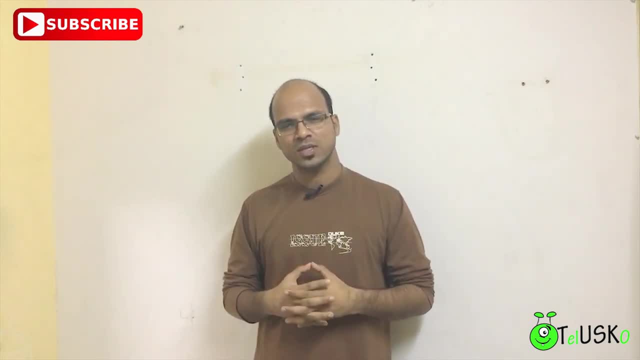 We'll take what you say assignment example in this. So let's imagine you have a school, Of course you're going to school or college, right. So in your school you'll be getting lots of assignments right and you need to complete the assignment and to complete the assignment. 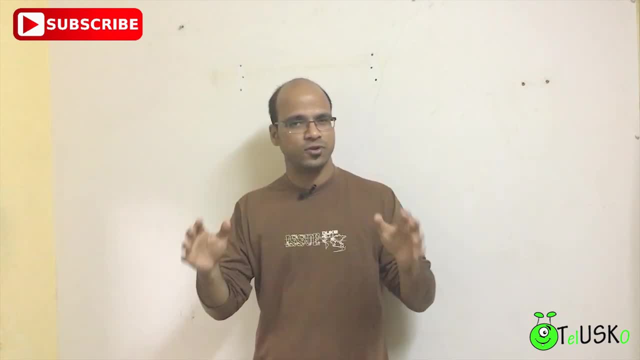 you have to do a assignment, right. You have to write your assignments. So that's a work for you, what we need- pen right. so your pen will be a property for the assignment work. so let's imagine you are doing assignment, you are writing your assignment, that's. 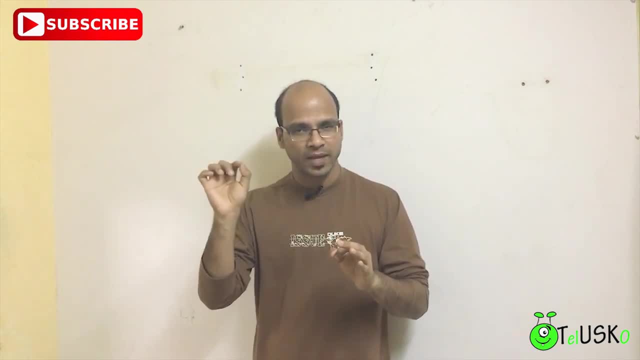 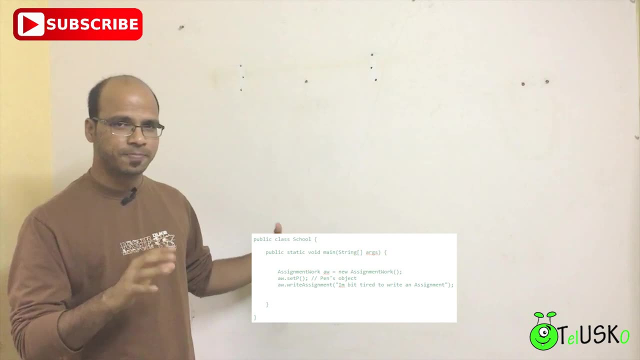 a method. so I write assignment is a method and to do that we require a pen, right? so in this example we have school and inside school, so that we have a main method there. so you have to write the assignment and we have a class which is assignment work, in which we'll be having a method which is write assignment. but 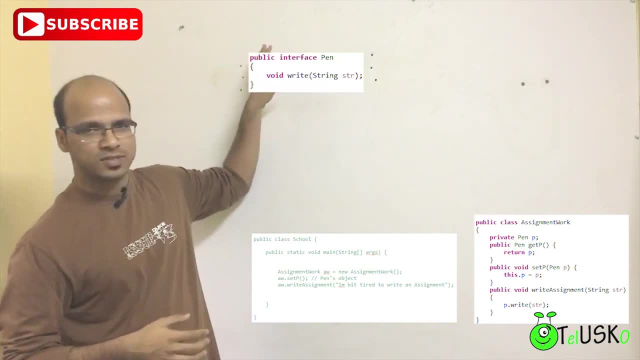 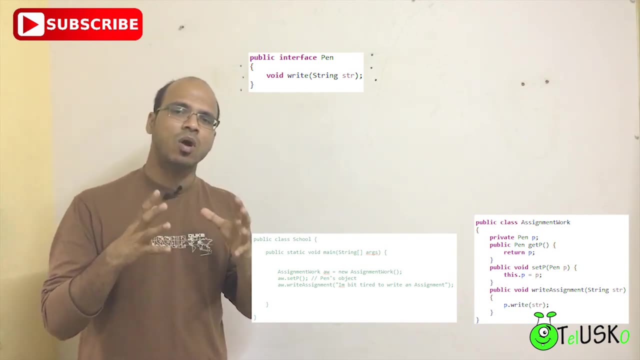 to write the assignment, we require a pen, right? so what is pen here? so pen is an interface. okay, so pen is an interface here, which is pen P, and also we have a pen there and that will be having a method. so in order to write the assignment, we require a pen, right? so let's imagine we have a pen property. 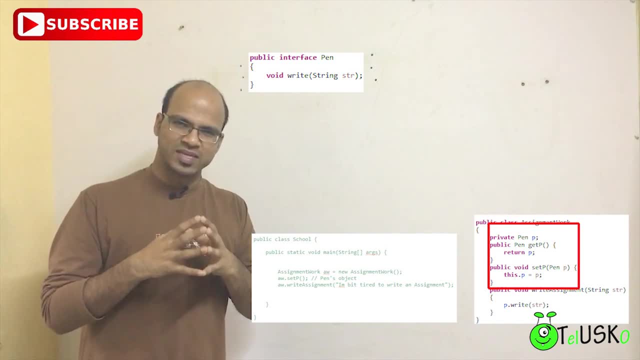 here. now. the problem is, once, when you want to write the assignment, you have to set the properties also. so you have a method, you have a setter there, you will set the pen, but we also need the implementation of pen, right? so we as a, as a developer, we have to create the implementation for pen, but hold on. 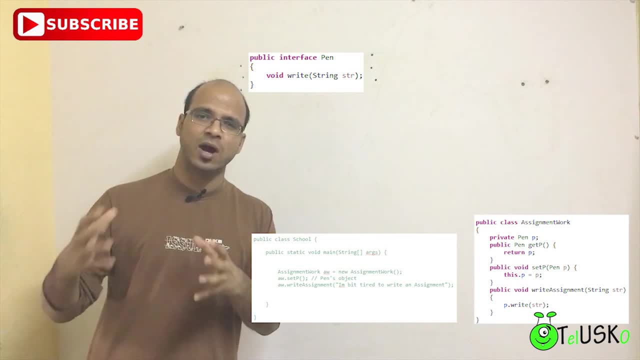 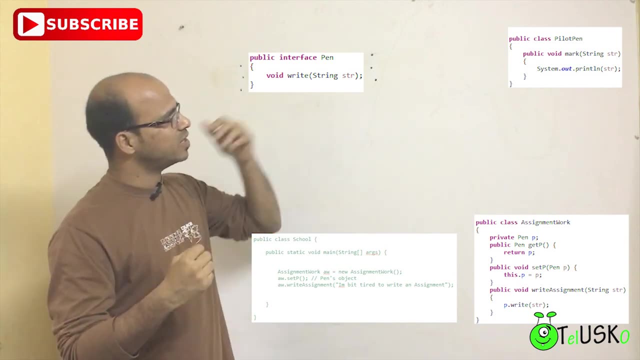 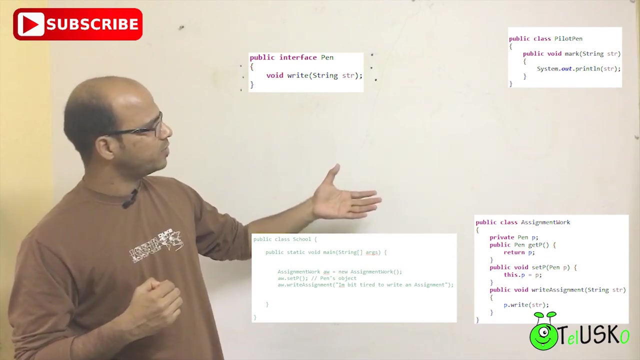 uh, I don't have the pen implementation, but I already have a pilot plan, pen implementation. so we have a pilot pen, so I have the implementation of pilot pen. okay, that's there. now how can you combine, how can you work with pilot pen here? because here you are mentioning pen, right, and we have a pen interface. we 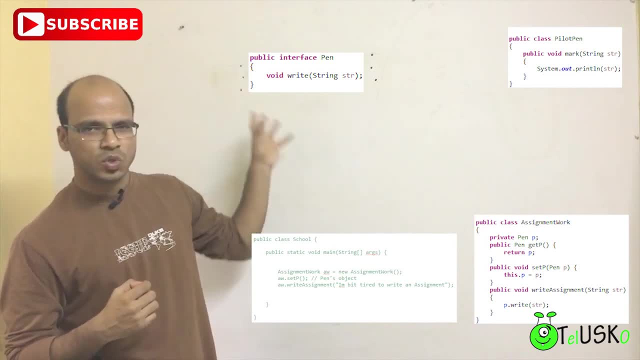 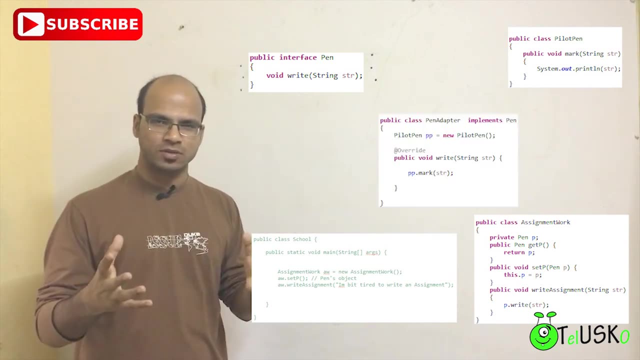 have a pilot pen class. so can we combine this two? can we use pilot pen in the place of pen directly? you cannot do that now here we need to use something called as adapter which will combine. so we'll be having a pen adapter which will take pilot pen object and it. 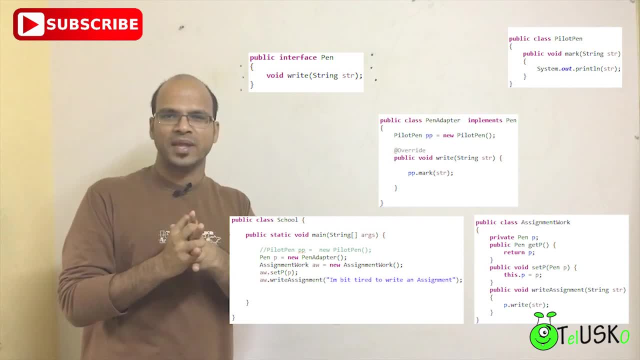 will provide pen object. I know how to do that. I will say in the practical implementation got the point right. so that's how you work with adapter design patterns provide the adapter between two different interfaces or two different classes. so to exactly do it, that will say in the practical. so if you like this, 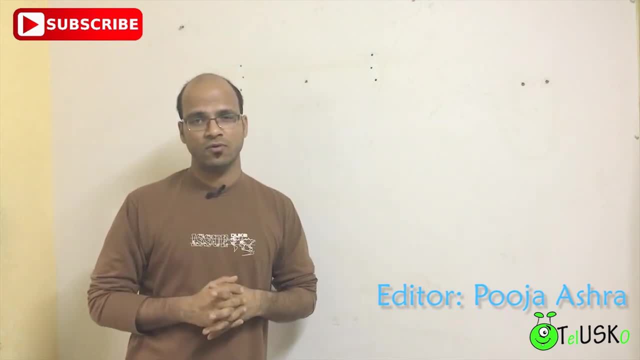 video. make sure you like the like the video and do subscribe for further video.